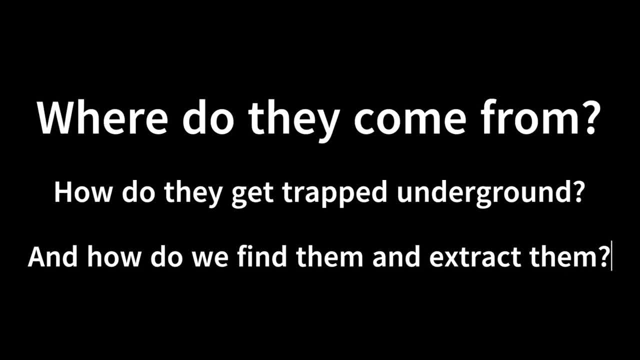 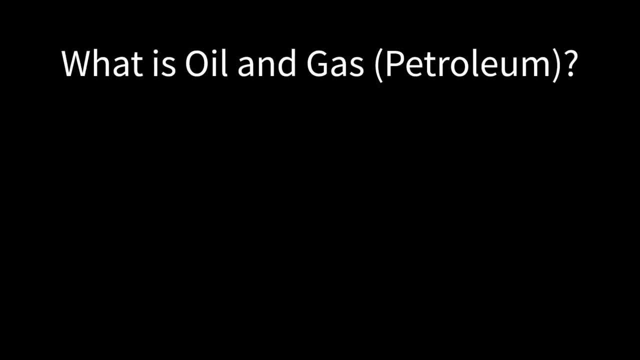 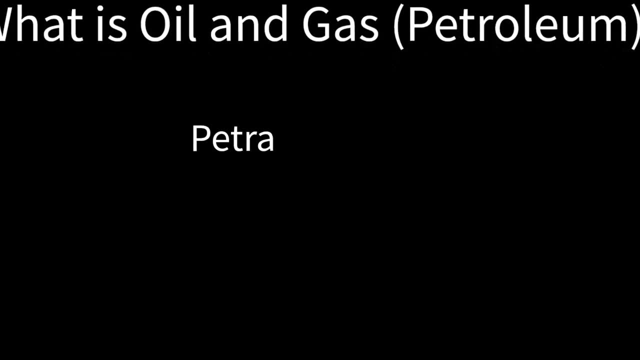 And how do we find them and extract them? If you want to learn more about the amazing world of petroleum geology, then keep watching. So what is oil and gas, or petroleum? Well, petroleum is derived from Latin words petra, meaning rock. 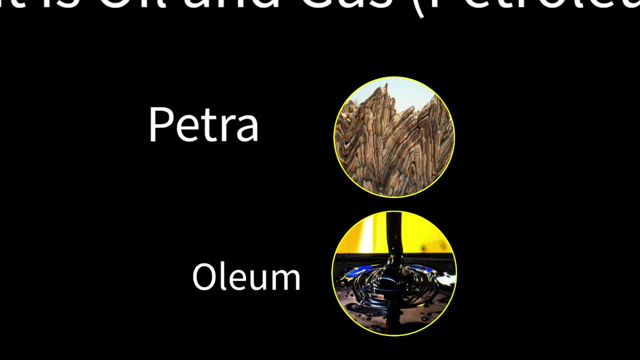 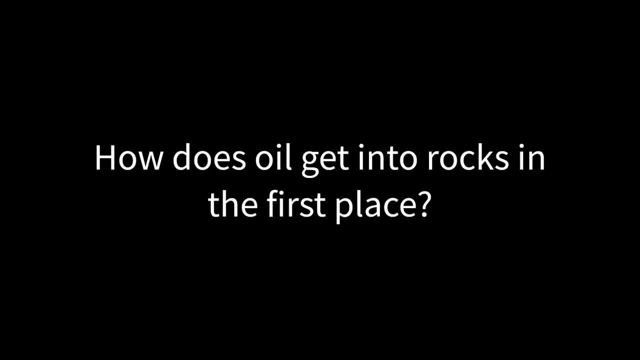 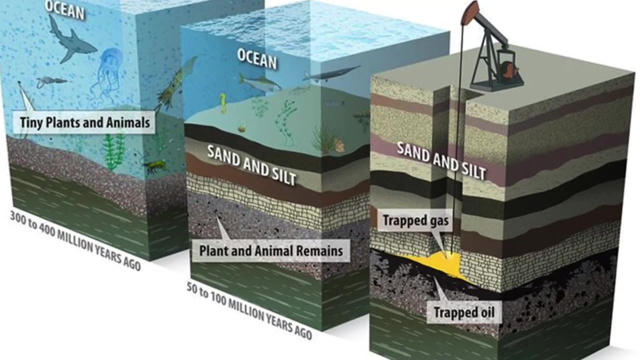 and oleum meaning oil. So to put it simply, petroleum is oil found in rock formations. But how does oil get into rocks in the first place? Oil and gas are actually formed from the remains of ancient plants and animals that lived millions of years ago. 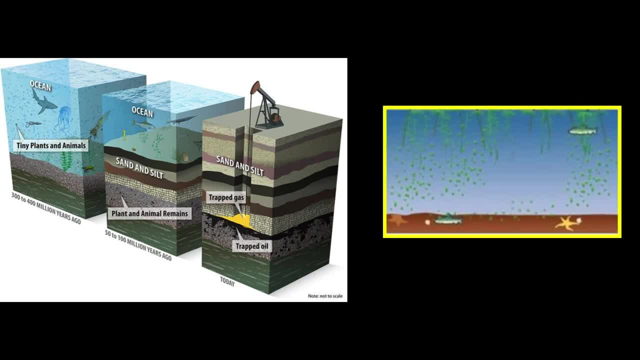 When these organisms died, they sank to the bottom of the oceans or lakes, where they were buried by layers of mud and silt. Over time, these layers became thicker and heavier, creating high pressure and temperature conditions that transformed the organic matter into hydrocarbons. 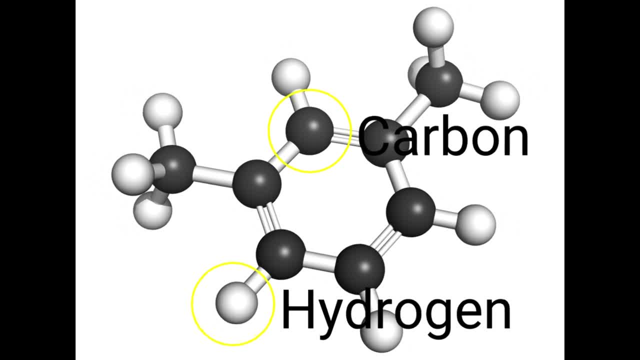 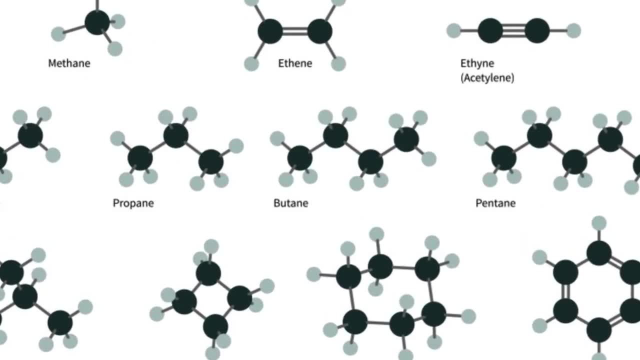 Hydrocarbons are molecules that consist only of carbon and hydrogen atoms. They can have different shapes inside. They can be of different sizes depending on how many carbon atoms they have and how they are arranged. For example, methane is the simplest hydrocarbon molecule. 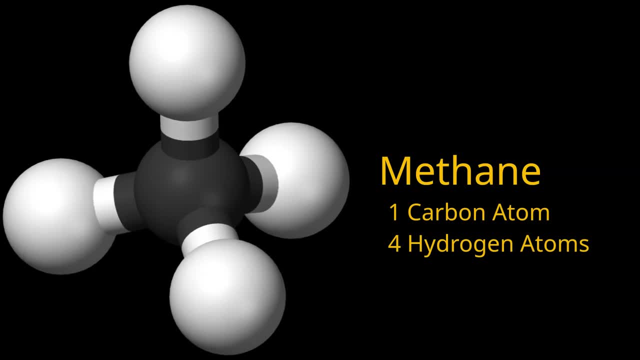 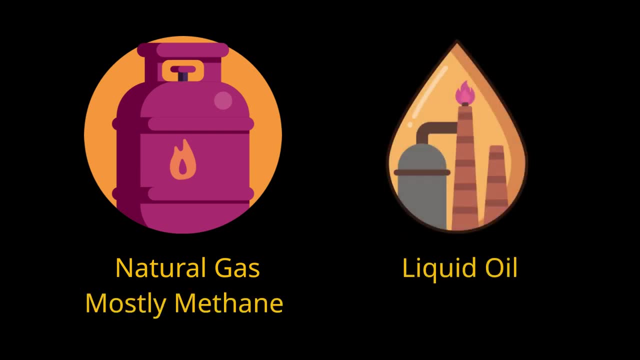 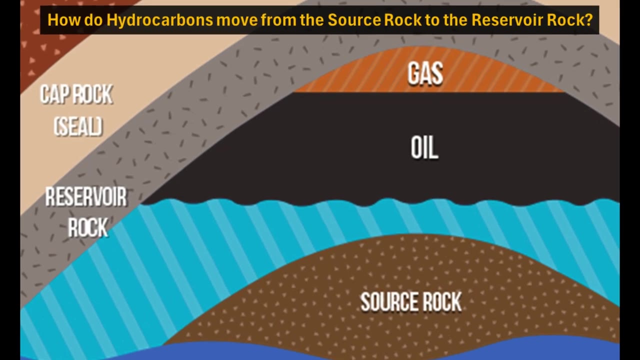 with one carbon atom joined to four hydrogen atoms. Hydrocarbons can occur as natural gas, which is mostly methane, or as liquid oil, which is a mixture of different hydrocarbons. But how do these hydrocarbons move from the source rock where they were formed, to the reservoir rock? 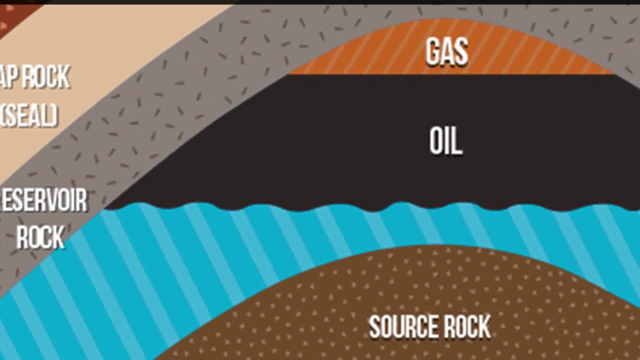 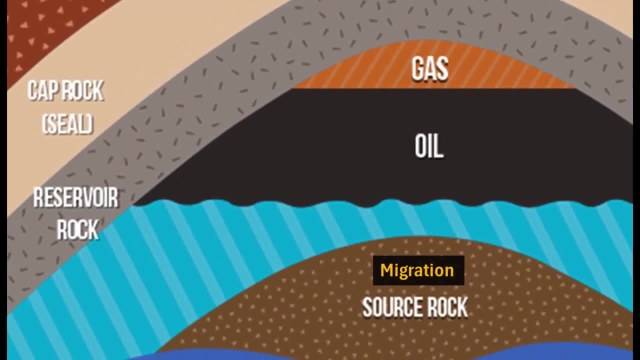 But how do these hydrocarbons move from the source rock, where they were formed, to the reservoir rock? But how do these hydrocarbons move from the source rock where they were formed to the reservoir rock? Well, this process is called migration, And it happens because hydrocarbons are lighter than water. 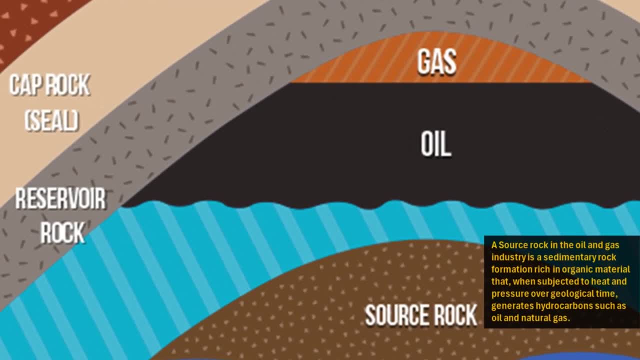 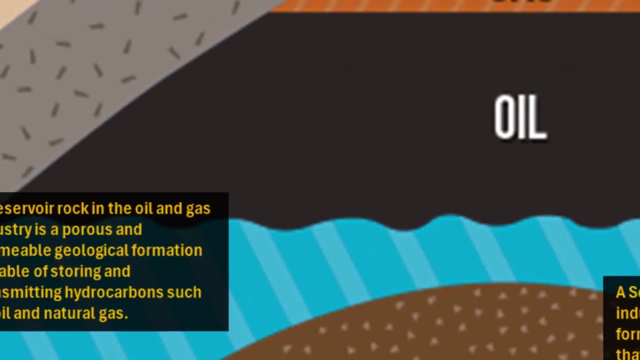 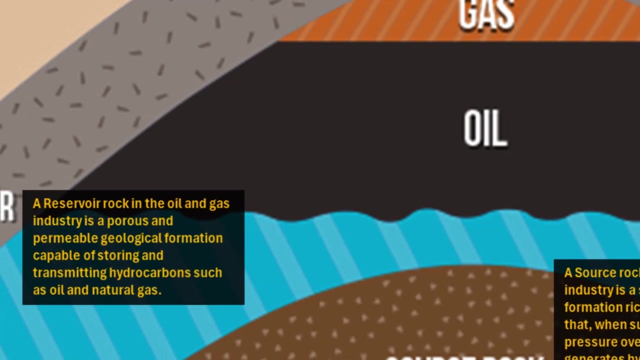 Oil and gas naturally want to rise upwards towards the surface through any porous and permeable rock formations that they encounter along the way. Porous means that the rock has spaces or pores between its grains or within its cracks or cavities. Permeable means that these pores are connected to the surface rock. 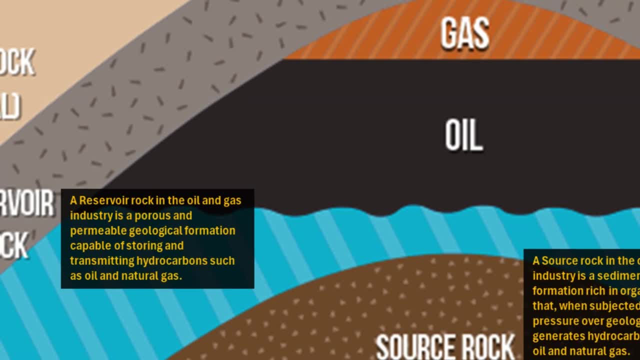 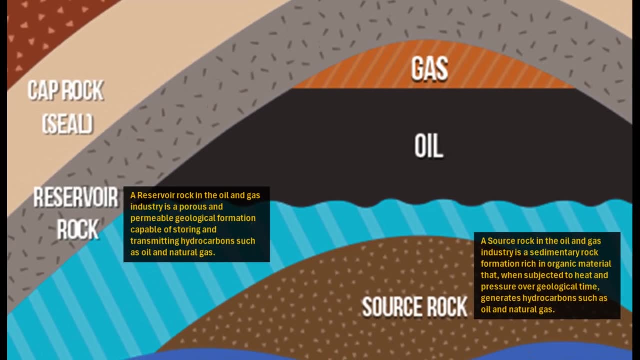 and they are connected and allow fluid to flow through them. The more porous and permeable a rock is, the more potential it has to hold hydrocarbons. But not all rocks are porous and permeable. Some rocks are impermeable, meaning that they block the flow of fluid. 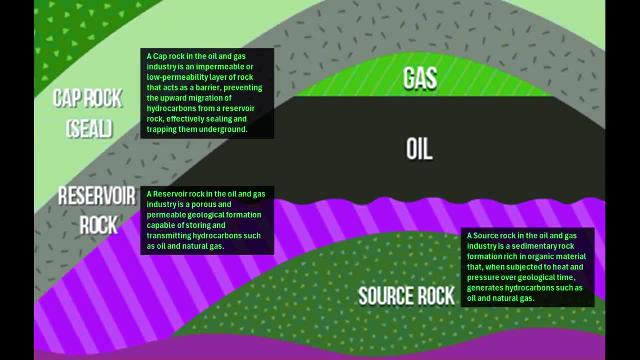 These rocks can act as seals or barriers that prevent oil and gas from escaping to the surface. When oil and gas encounter an impermeable rock layer above a porous and permeable rock layer. When oil and gas encounter an impermeable rock layer above a porous and permeable rock layer. 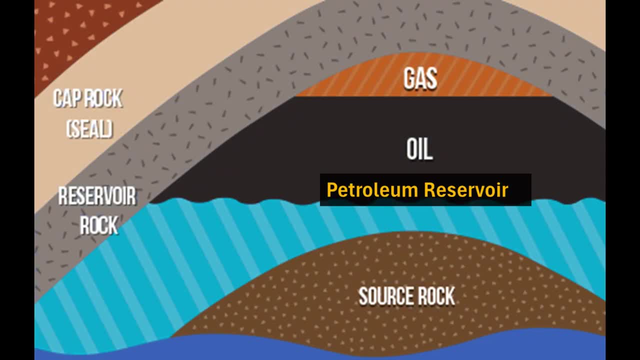 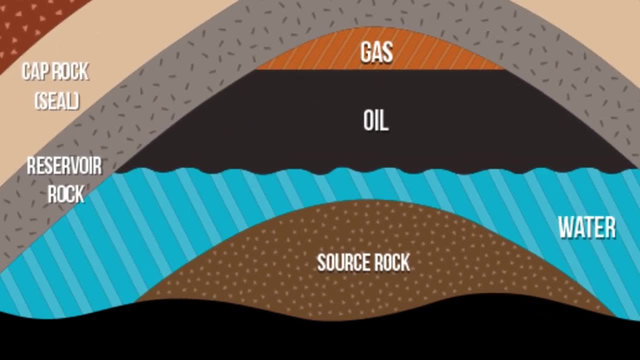 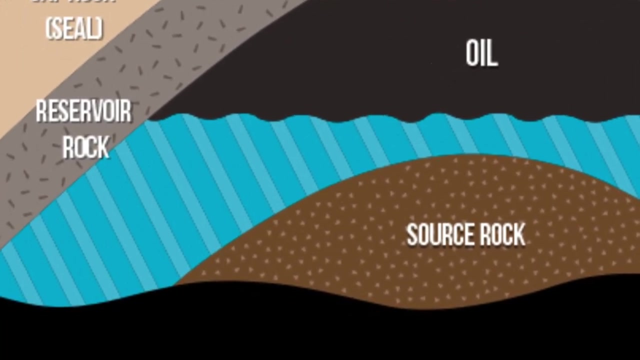 they get trapped in a subsurface pool called a petroleum reservoir. But not all reservoirs are created equal. There are different types of traps that can form a reservoir, depending on the shape and structure of the rock layers. Let's look at some examples. 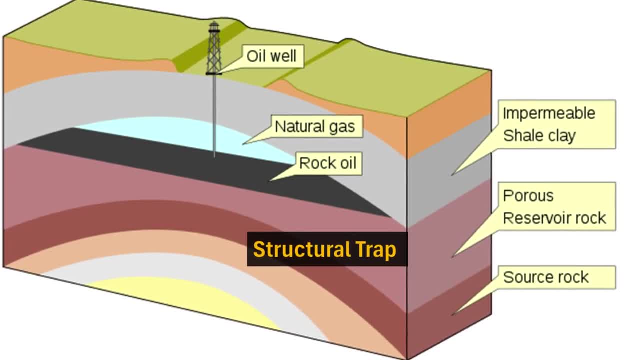 One type of trap is called a structural trap. This is when the rock layers are deformed or displaced by tectonic forces such as folding or faulting. This is when the rock layers are deformed or displaced by tectonic forces such as folding or faulting. 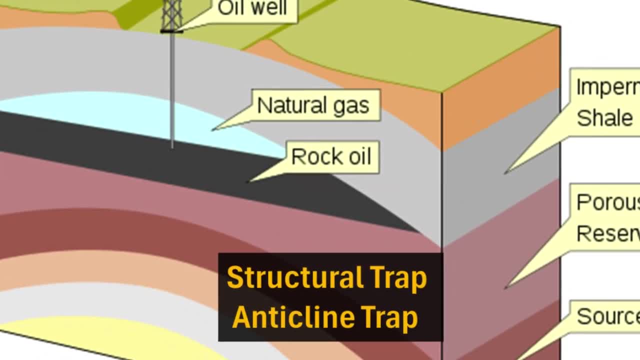 For example, an anticline trap is an upward fold of the layers of rock. For example, an anticline trap is an upward fold of the layers of rock. Oil and gas migrate into the highest part of the fold, where they are trapped by an overlying impermeable layer. 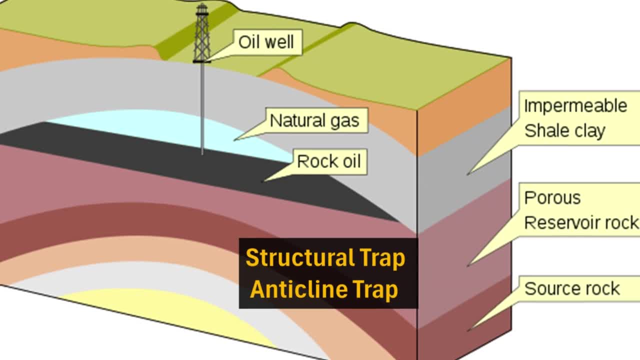 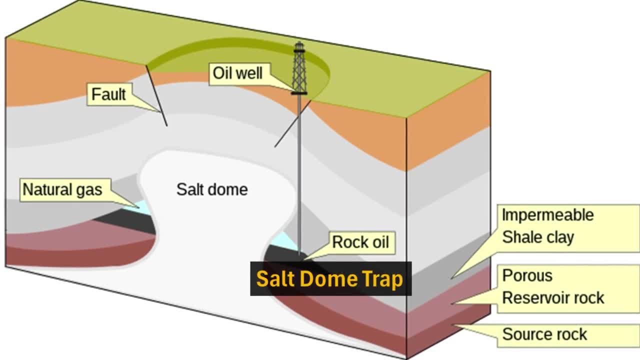 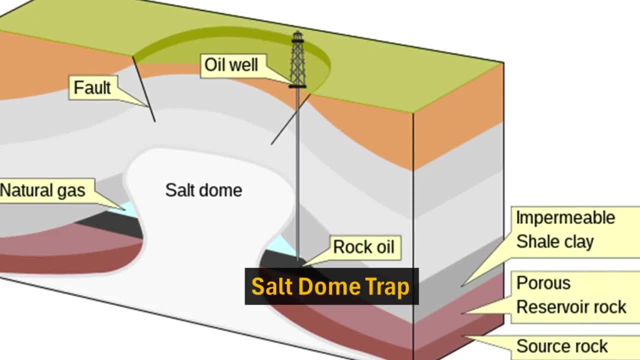 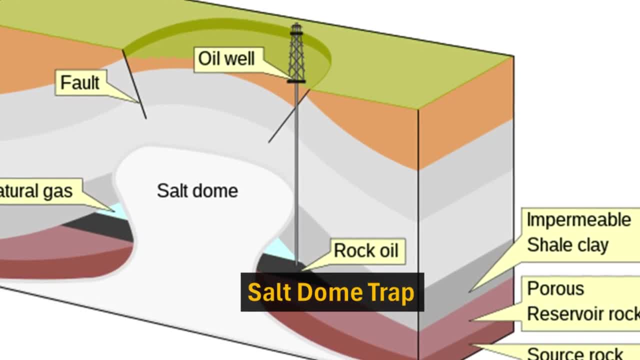 As it rises, it pushes aside and breaks through many layers of rock in its path. As it rises, it pushes aside and breaks through many layers of rock in its path. If it encounters a porous and permeable layer that contains oil and gas, it can create a trap by sealing it off with its impermeable salt. 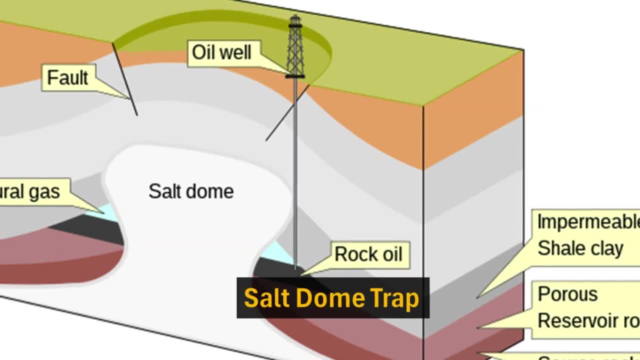 If it encounters a porous and permeable layer that contains oil and gas, it can create a trap by sealing it off with its impermeable salt. If it encounters a porous and permeable layer that contains oil and gas, it can create a trap by sealing it off with its impermeable salt. 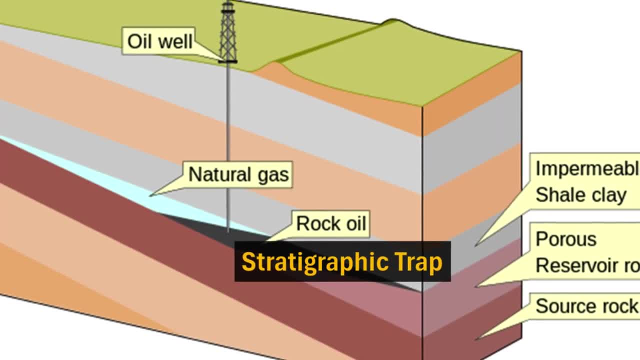 If it encounters a porous and permeable layer that contains oil and gas, it can create a trap by sealing it off with its impermeable salt. If it encounters a porous and permeable layer that contains oil and gas, it can create a trap by sealing it off with its impermeable salt. 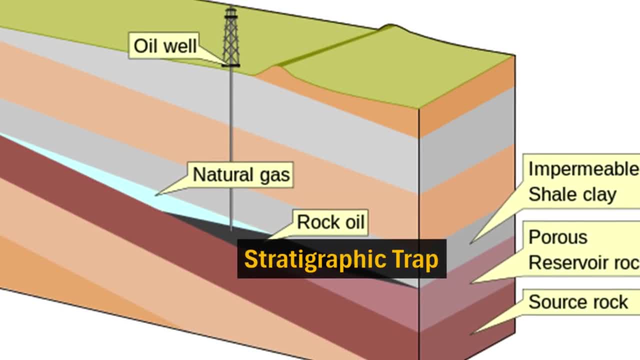 If it encounters a porous and permeable layer that contains oil and gas, it can create a trap by sealing it off with its impermeable salt. If it encounters a porous and permeable layer that contains oil and gas, it can create a trap by sealing it off with its impermeable salt. 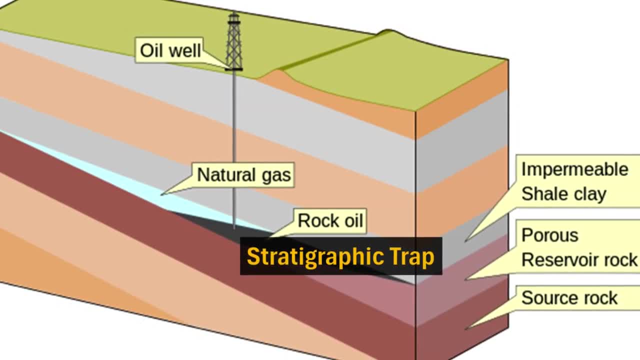 If it encounters a porous and permeable layer that contains oil and gas, it can create a trap by sealing it off with its impermeable salt. If it encounters a porous and permeable layer that contains oil and gas, it can create a trap by sealing it off with its impermeable salt. 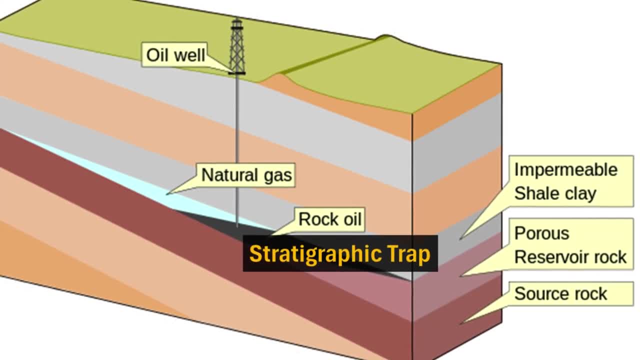 If it encounters a porous and permeable layer that contains oil and gas, it can create a trap by sealing it off with its impermeable salt. If it encounters a porous and permeable layer that contains oil and gas, it can create a trap by sealing it off with its impermeable salt. 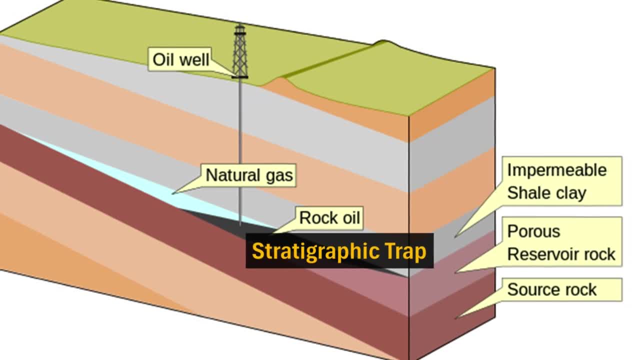 If it encounters a porous and permeable layer that contains oil and gas, it can create a trap by sealing it off with its impermeable salt. If it encounters a porous and permeable layer that contains oil and gas, it can create a trap by sealing it off with its impermeable salt. 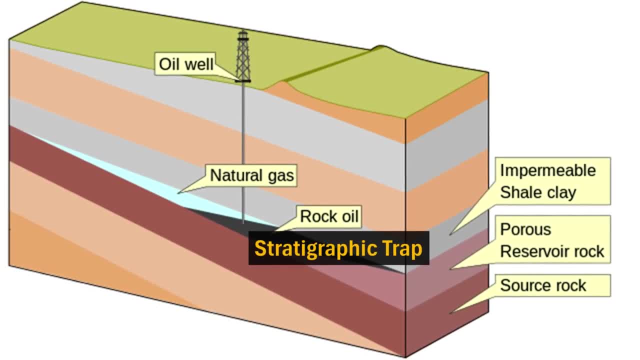 If it encounters a porous and permeable layer that contains oil and gas, it can create a trap by sealing it off with its impermeable salt. If it encounters a porous and permeable layer that contains oil and gas, it can create a trap by sealing it off with its impermeable salt. 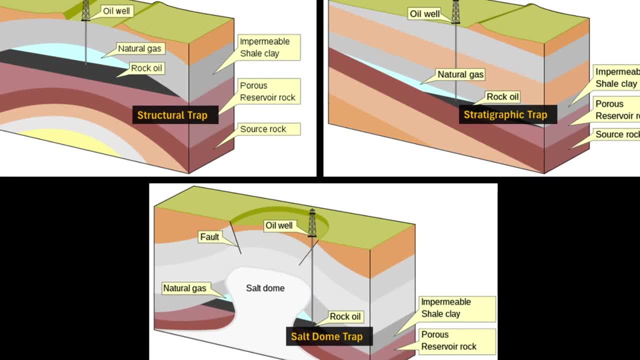 If it encounters a porous and permeable layer that contains oil and gas, it can create a trap by sealing it off with its impermeable salt. If it encounters a porous and permeable layer that contains oil and gas, it can create a trap by sealing it off with its impermeable salt. 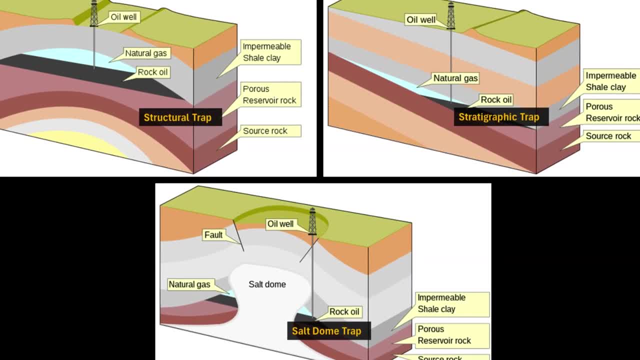 If it encounters a porous and permeable layer that contains oil and gas, it can create a trap by sealing it off with its impermeable salt. If it encounters a porous and permeable layer that contains oil and gas, it can create a trap by sealing it off with its impermeable salt. 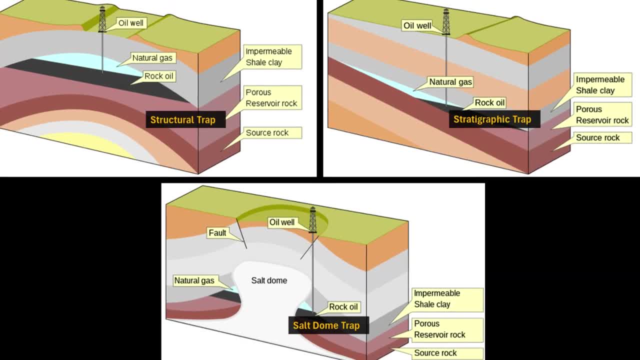 If it encounters a porous and permeable layer that contains oil and gas, it can create a trap by sealing it off with its impermeable salt. If it encounters a porous and permeable layer that contains oil and gas, it can create a trap by sealing it off with its impermeable salt. 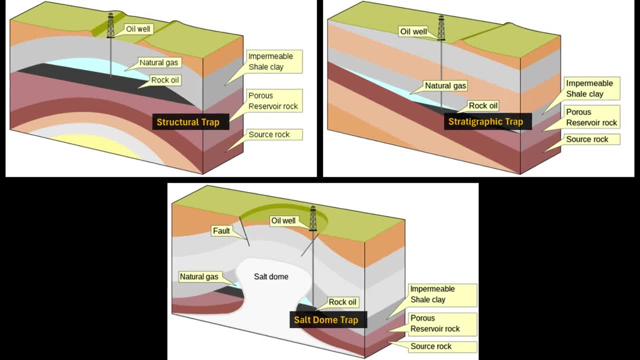 If it encounters a porous and permeable layer that contains oil and gas, it can create a trap by sealing it off with its impermeable salt. If it encounters a porous and permeable layer that contains oil and gas, it can create a trap by sealing it off with its impermeable salt. 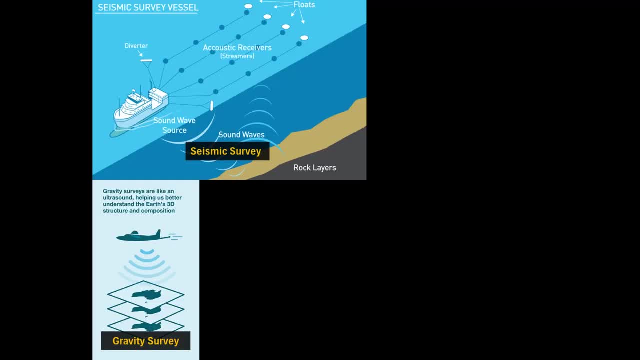 If it encounters a porous and permeable layer that contains oil and gas, it can create a trap by sealing it off with its impermeable salt. If it encounters a porous and permeable layer that contains oil and gas, it can create a trap by sealing it off with its impermeable salt. 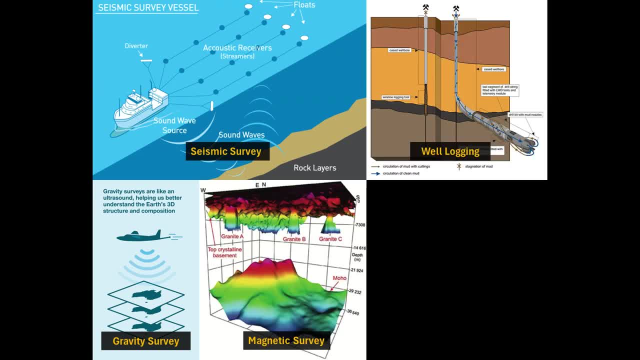 If it encounters a porous and permeable layer that contains oil and gas, it can create a trap by sealing it off with its impermeable salt. If it encounters a porous and permeable layer that contains oil and gas, it can create a trap by sealing it off with its impermeable salt. 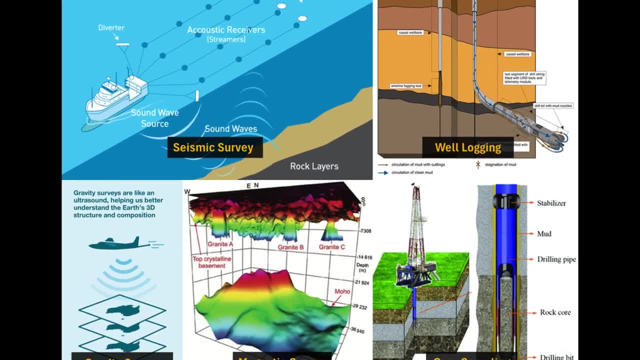 If it encounters a porous and permeable layer that contains oil and gas, it can create a trap by sealing it off with its impermeable salt. If it encounters a porous and permeable layer that contains oil and gas, it can create a trap by sealing it off with its impermeable salt. 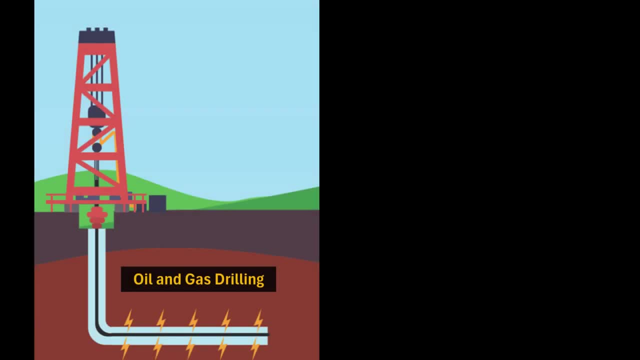 If it encounters a porous and permeable layer that contains oil and gas, it can create a trap by sealing it off with its impermeable salt. If it encounters a porous and permeable layer that contains oil and gas, it can create a trap by sealing it off with its impermeable salt. 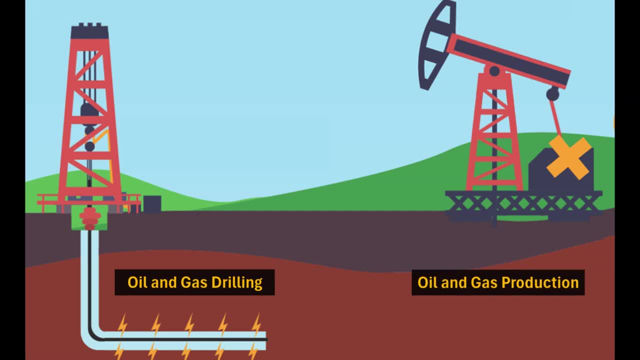 If it encounters a porous and permeable layer that contains oil and gas, it can create a trap by sealing it off with its impermeable salt. If it encounters a porous and permeable layer that contains oil and gas, it can create a trap by sealing it off with its impermeable salt. 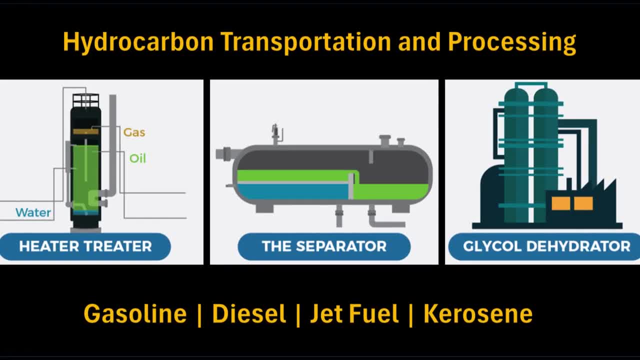 If it encounters a porous and permeable layer that contains oil and gas, it can create a trap by sealing it off with its impermeable salt. If it encounters a porous and permeable layer that contains oil and gas, it can create a trap by sealing it off with its impermeable salt. 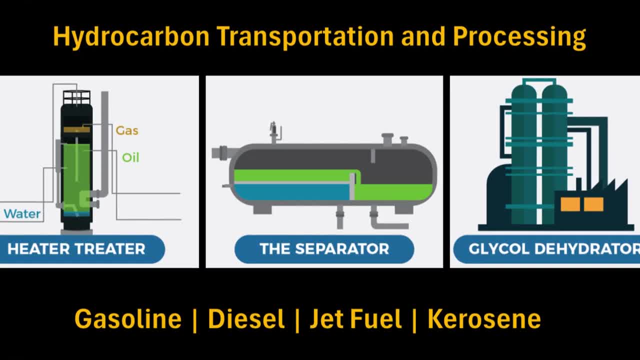 If it encounters a porous and permeable layer that contains oil and gas, it can create a trap by sealing it off with its impermeable salt. If it encounters a porous and permeable layer that contains oil and gas, it can create a trap by sealing it off with its impermeable salt. 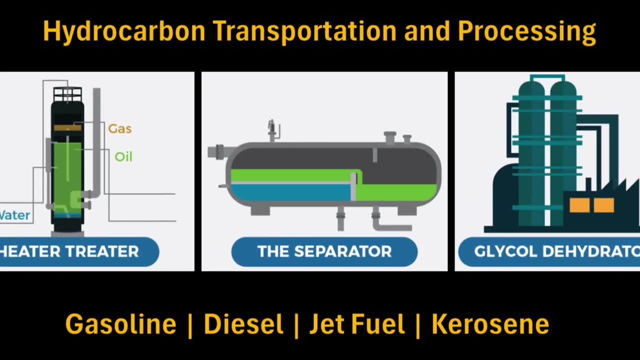 If it encounters a porous and permeable layer that contains oil and gas, it can create a trap by sealing it off with its impermeable salt. If it encounters a porous and permeable layer that contains oil and gas, it can create a trap by sealing it off with its impermeable salt. 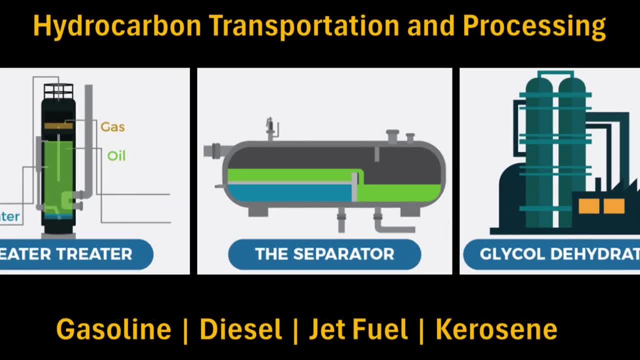 If it encounters a porous and permeable layer that contains oil and gas, it can create a trap by sealing it off with its impermeable salt. If it encounters a porous and permeable layer that contains oil and gas, it can create a trap by sealing it off with its impermeable salt. 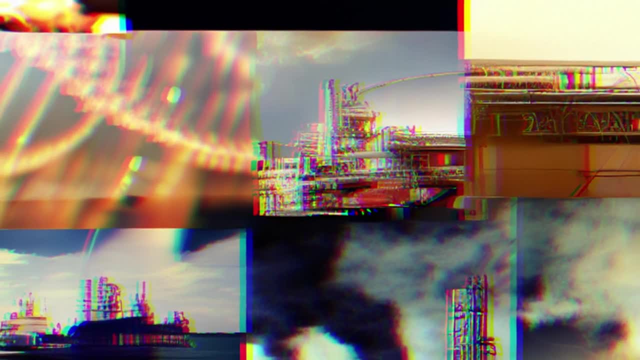 If it encounters a porous and permeable layer that contains oil and gas, it can create a trap by sealing it off with its impermeable salt. If it encounters a porous and permeable layer that contains oil and gas, it can create a trap by sealing it off with its impermeable salt. 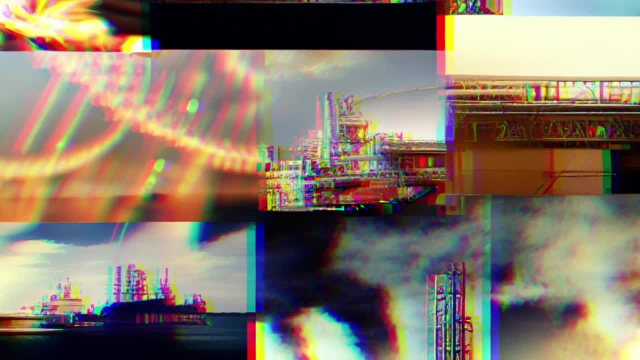 If it encounters a porous and permeable layer that contains oil and gas, it can create a trap by sealing it off with its impermeable salt. If it encounters a porous and permeable layer that contains oil and gas, it can create a trap by sealing it off with its impermeable salt. 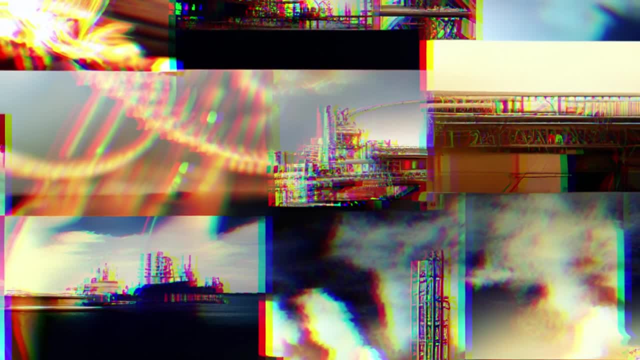 If it encounters a porous and permeable layer that contains oil and gas, it can create a trap by sealing it off with its impermeable salt. If it encounters a porous and permeable layer that contains oil and gas, it can create a trap by sealing it off with its impermeable salt. 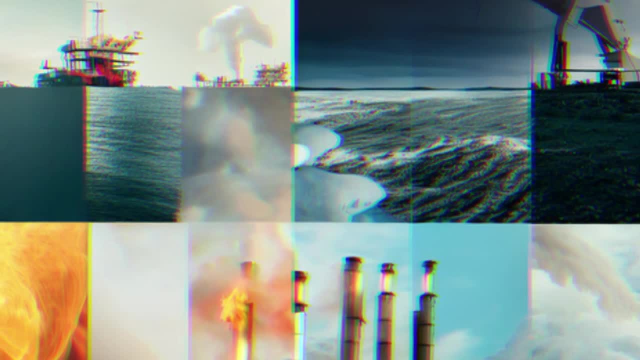 If it encounters a porous and permeable layer that contains oil and gas, it can create a trap by sealing it off with its impermeable salt. If it encounters a porous and permeable layer that contains oil and gas, it can create a trap by sealing it off with its impermeable salt. 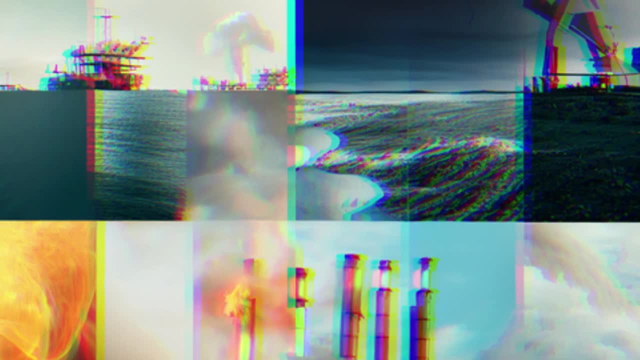 If it encounters a porous and permeable layer that contains oil and gas, it can create a trap by sealing it off with its impermeable salt. If it encounters a porous and permeable layer that contains oil and gas, it can create a trap by sealing it off with its impermeable salt. 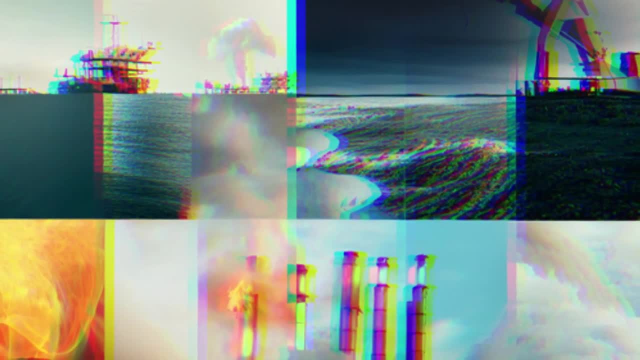 If it encounters a porous and permeable layer that contains oil and gas, it can create a trap by sealing it off with its impermeable salt. If it encounters a porous and permeable layer that contains oil and gas, it can create a trap by sealing it off with its impermeable salt. 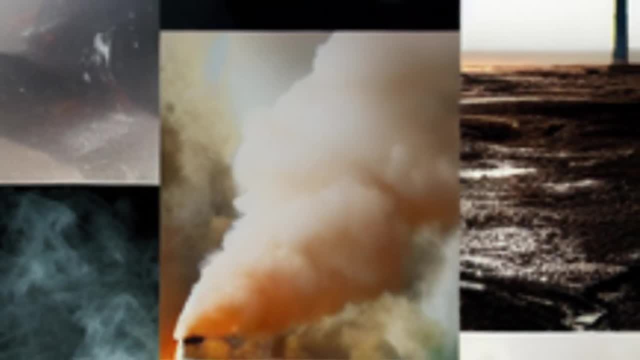 If it encounters a porous and permeable layer that contains oil and gas, it can create a trap by sealing it off with its impermeable salt. If it encounters a porous and permeable layer that contains oil and gas, it can create a trap by sealing it off with its impermeable salt. 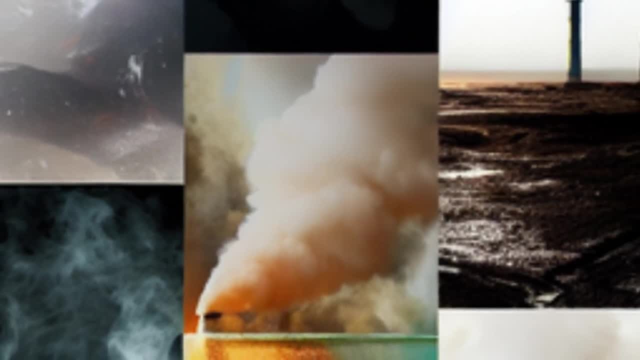 If it encounters a porous and permeable layer that contains oil and gas, it can create a trap by sealing it off with its impermeable salt. If it encounters a porous and permeable layer that contains oil and gas, it can create a trap by sealing it off with its impermeable salt. 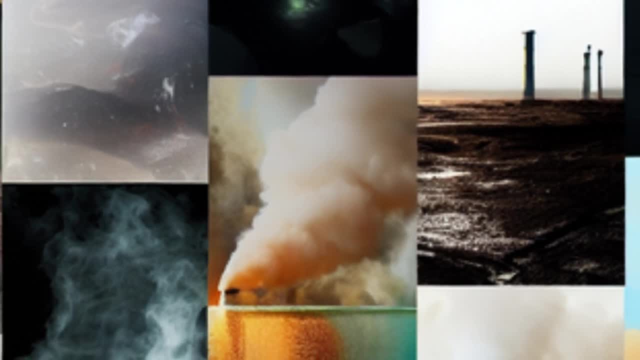 If it encounters a porous and permeable layer that contains oil and gas, it can create a trap by sealing it off with its impermeable salt. If it encounters a porous and permeable layer that contains oil and gas, it can create a trap by sealing it off with its impermeable salt. 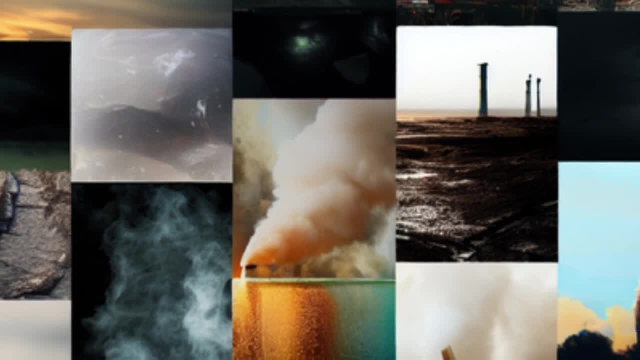 If it encounters a porous and permeable layer that contains oil and gas, it can create a trap by sealing it off with its impermeable salt. If it encounters a porous and permeable layer that contains oil and gas, it can create a trap by sealing it off with its impermeable salt. 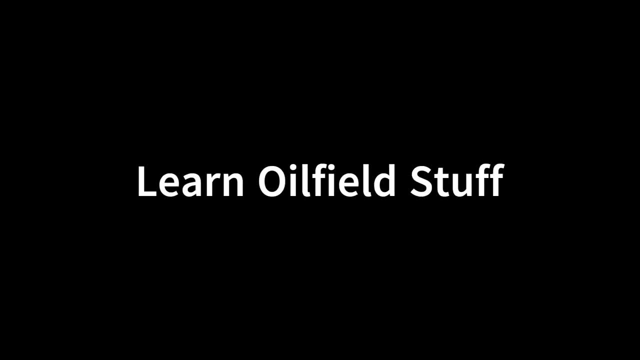 If it encounters a porous and permeable layer that contains oil and gas, it can create a trap by sealing it off with its impermeable salt. If it encounters a porous and permeable layer that contains oil and gas, it can create a trap by sealing it off with its impermeable salt. 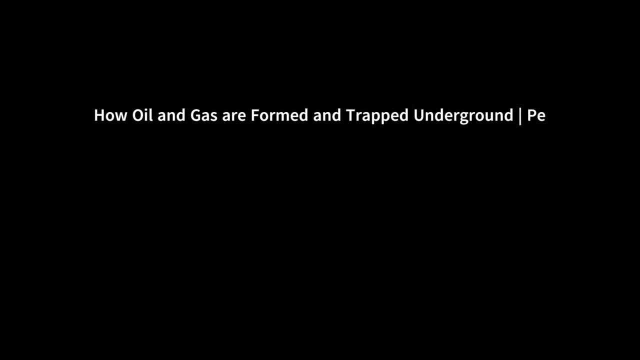 If it encounters a porous and permeable layer that contains oil and gas, it can create a trap by sealing it off with its impermeable salt. If it encounters a porous and permeable layer that contains oil and gas, it can create a trap by sealing it off with its impermeable salt. 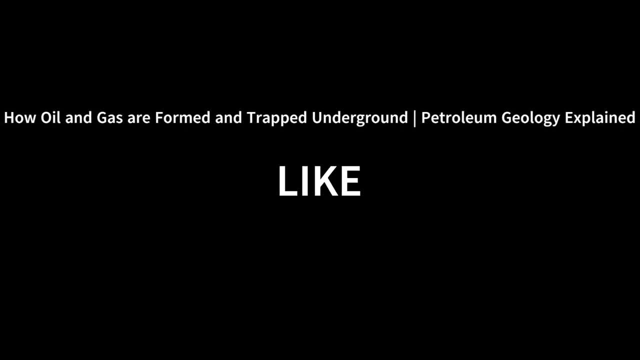 If it encounters a porous and permeable layer that contains oil and gas, it can create a trap by sealing it off with its impermeable salt. If it encounters a porous and permeable layer that contains oil and gas, it can create a trap by sealing it off with its impermeable salt. 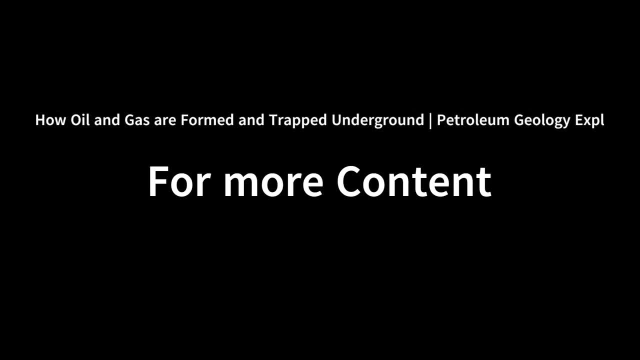 If it encounters a porous and permeable layer that contains oil and gas, it can create a trap by sealing it off with its impermeable salt. If it encounters a porous and permeable layer that contains oil and gas, it can create a trap by sealing it off with its impermeable salt. 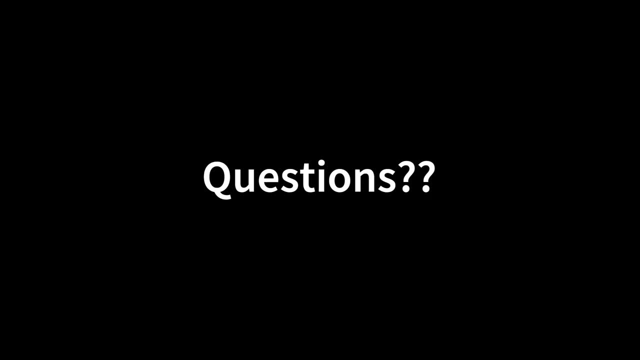 If it encounters a porous and permeable layer that contains oil and gas, it can create a trap by sealing it off with its impermeable salt. If it encounters a porous and permeable layer that contains oil and gas, it can create a trap by sealing it off with its impermeable salt. 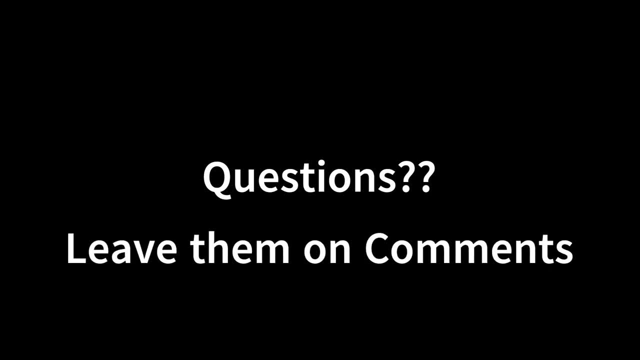 If it encounters a porous and permeable layer that contains oil and gas, it can create a trap by sealing it off with its impermeable salt. If it encounters a porous and permeable layer that contains oil and gas, it can create a trap by sealing it off with its impermeable salt. 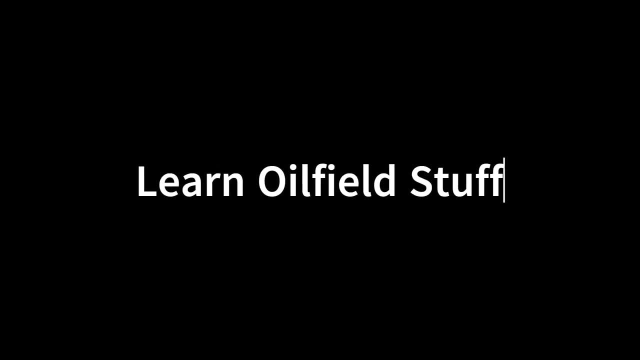 If it encounters a porous and permeable layer that contains oil and gas, it can create a trap by sealing it off with its impermeable salt. If it encounters a porous and permeable layer that contains oil and gas, it can create a trap by sealing it off with its impermeable salt.